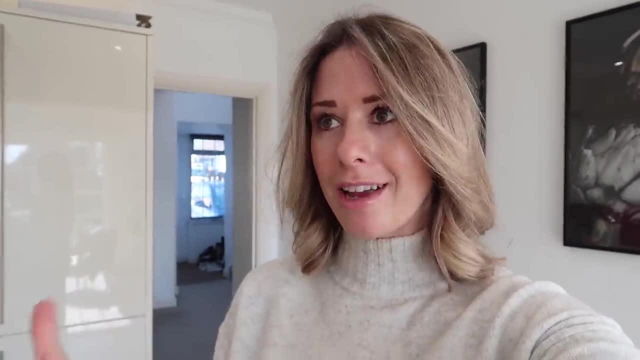 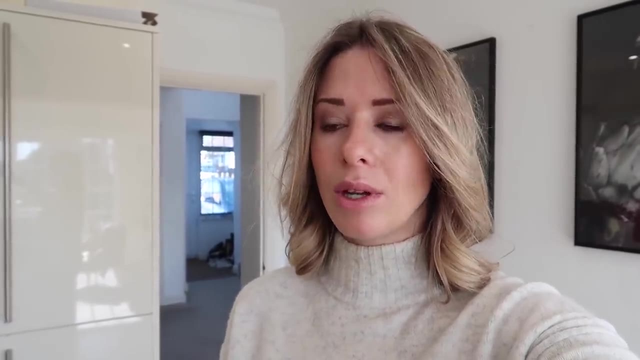 pick up a couple of extra items, like extra things to put in the freezer or extra tins in case we go into lockdown, because obviously then going out and about is not recommended. So we just thought, if we can be as prepared as we can do, we're not one of those people who are like panic buying at 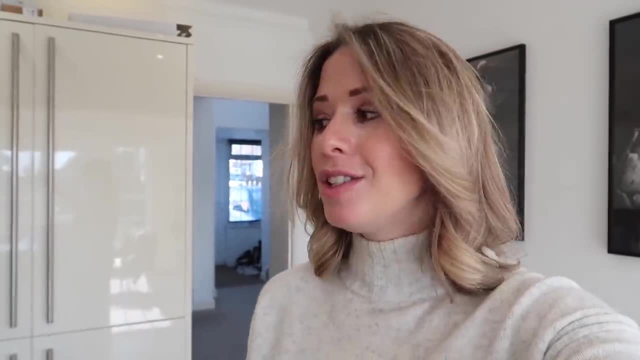 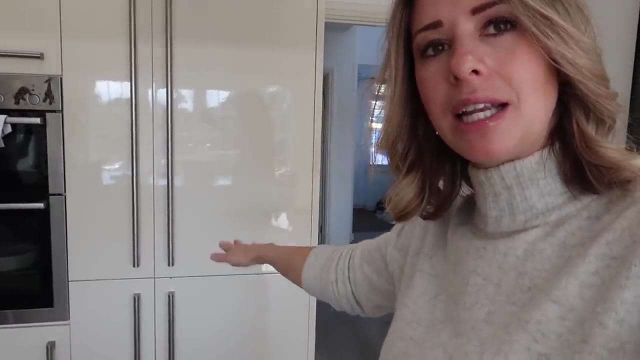 all. We're just being a little bit more prepared than we normally would be. So we have got two 30% freezers. So you know, when you have like a fridge freezer like this, that is 70% and it's the fridge. 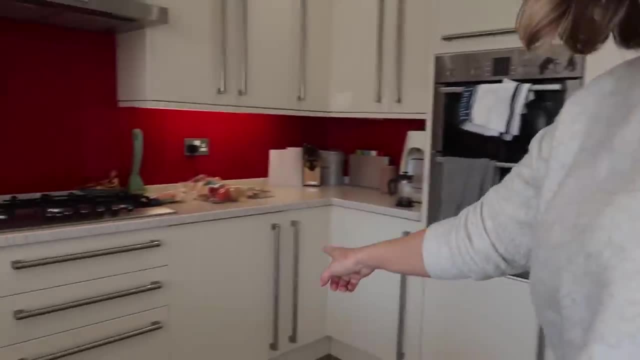 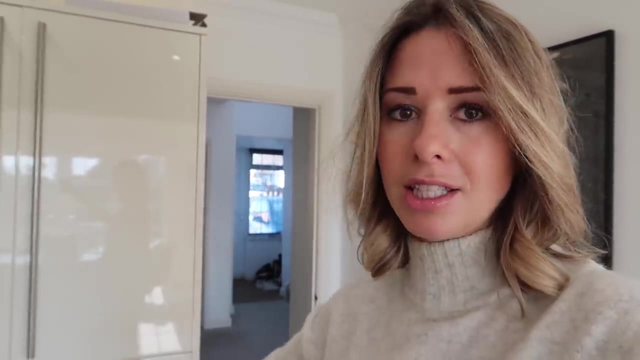 and then that is 30% and it's the freezer. So we've got one of those there and we've got another one there, which we're very lucky to have, because in our old house we only had the one like fridge freezer: 70, 30%. So today I'm just going to show you what we are going to be doing to our fridge. 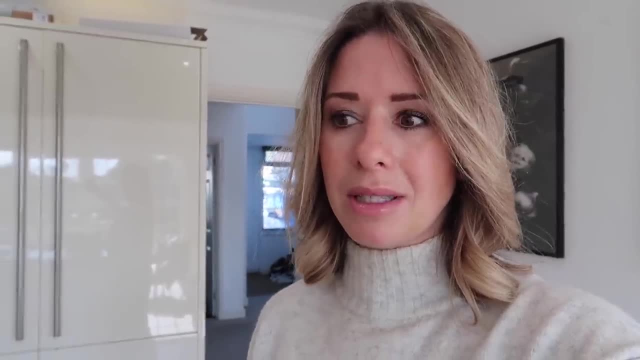 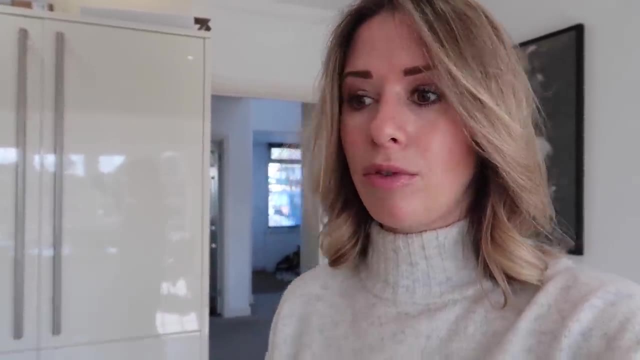 freezers to maximise the space. We've been living in this house for about six months now and we haven't ever defrosted our freezers. There's quite a lot of ice buildup on them. And then, obviously, the people who own this house before us. I'm not sure when they last. 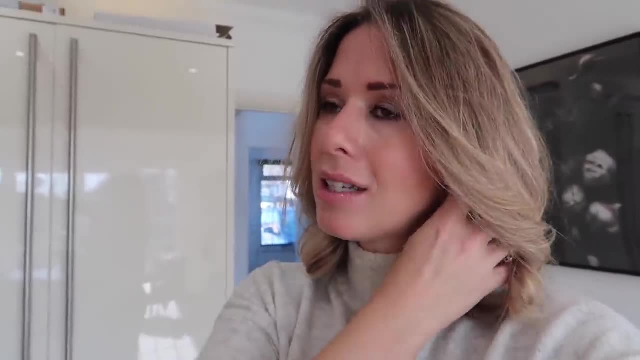 defrosted them either. So I'm going to show you what we have in our two freezers And also. Chris has just been to the shop now as well. He's bought a couple of extra bits as well which don't fit in. 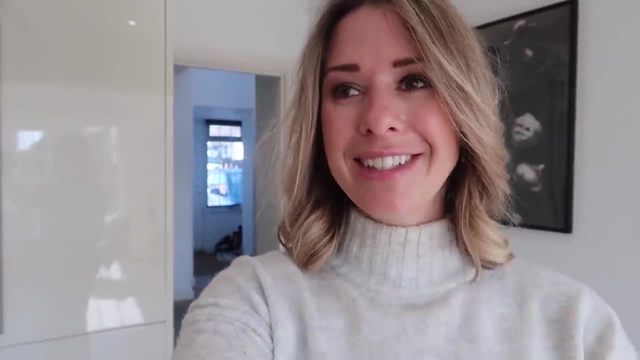 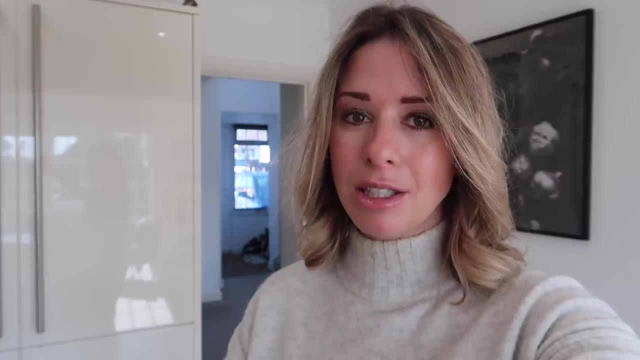 the freezer at the moment, which is why I wanted to make this video. So Chris has said very kindly that he will be the one who defrosts our freezers for us. So what I'm going to do is get some of the ice in our freezers, put them into a cool bag and then put all of our frozen food into that cool 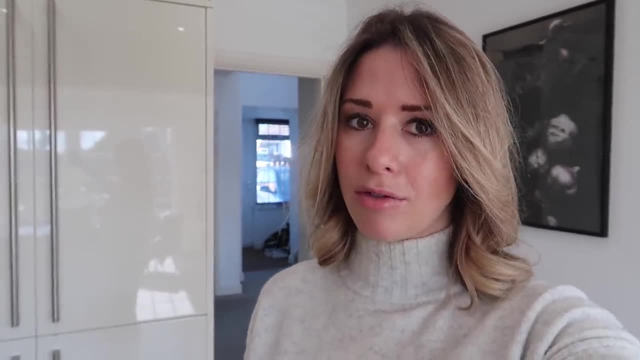 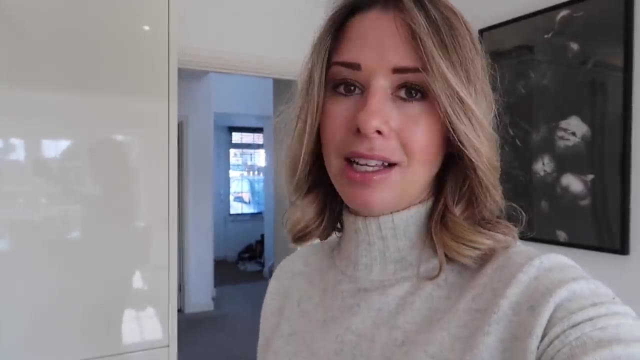 bag to keep it nice and cold and frozen whilst we are defrosting. Basically, what we're going to do to defrost is chip off all the ice that has built up in the fridge, And then it's just going to give us so much more space, because I'm going to show you now how many centimetres the ice is taking up. 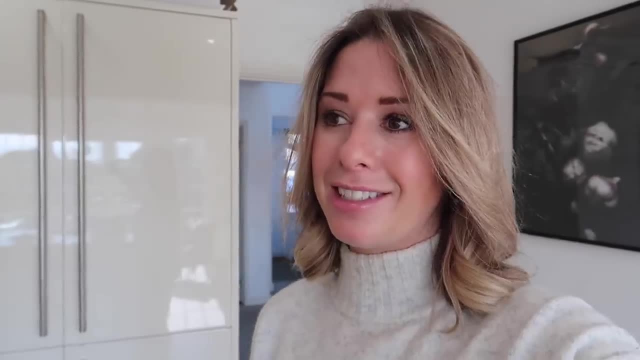 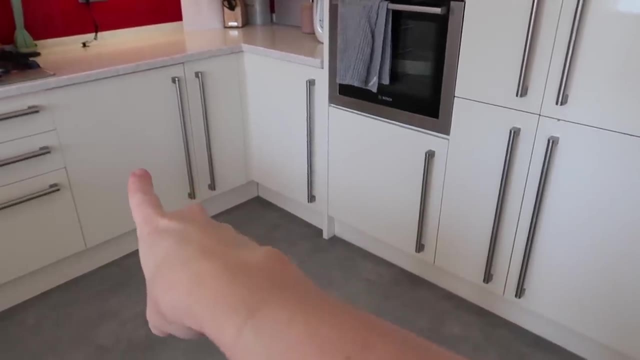 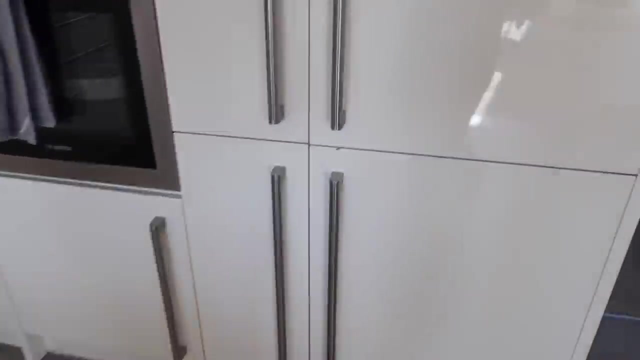 in our freezer. So let's get going. Chris is even in his gym gear to do this. Let's do it Right. And then there as well. So we are quite lucky, because in our old house we only had that one freezer. So it means we've been able to kind of like, kind of over time, stocked up a little bit. 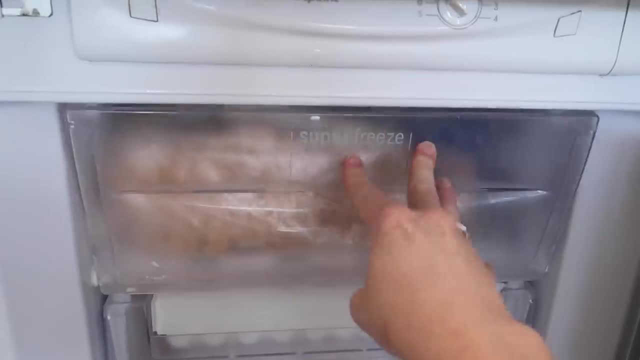 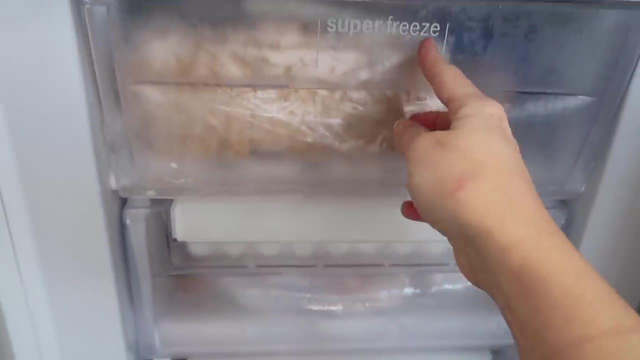 more. But, as you can see, like I can't even shut that top one because it's just so full, And I feel like if I scraped away all of this ice and defrosted the whole freezer properly, then I'd be able to fit so much more in. So I've still got all of this in here without putting everything. 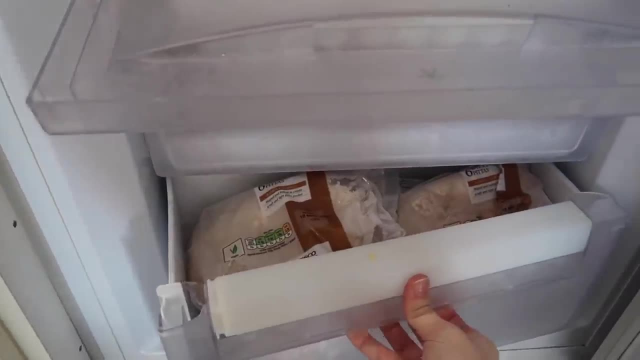 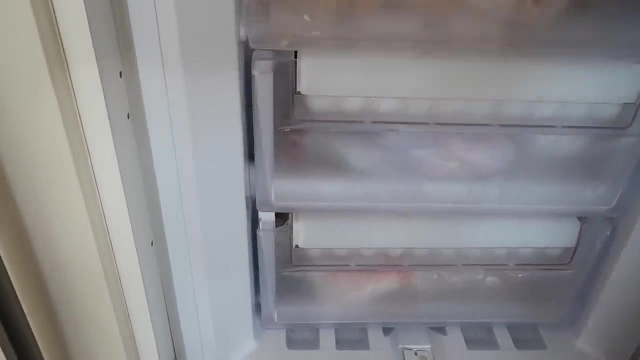 else, like the pizzas that I've got in here As well. So I'm stocked up quite a bit of bread because that's always great to kind of have in your freezer to last you. But, like I said, that doesn't close, So I have to kind of hold it up. 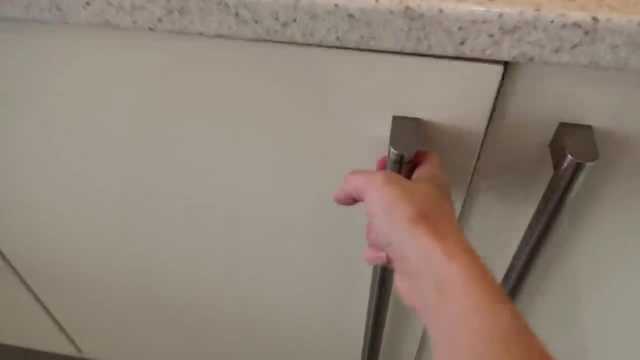 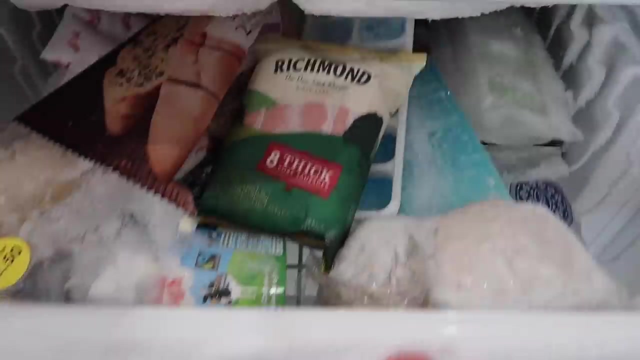 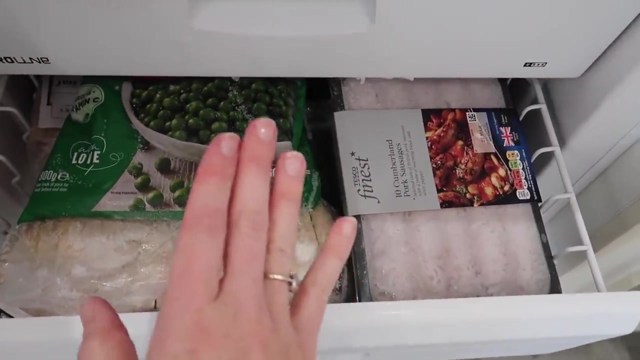 while I shut the freezer over here. You can see there's been quite a lot like ice build up here and up there, So these are quite full as well. already I've got lots of ice packs in here, So these are what I'm actually going to use. Loads of sausages. I've got more bread, more bread there. 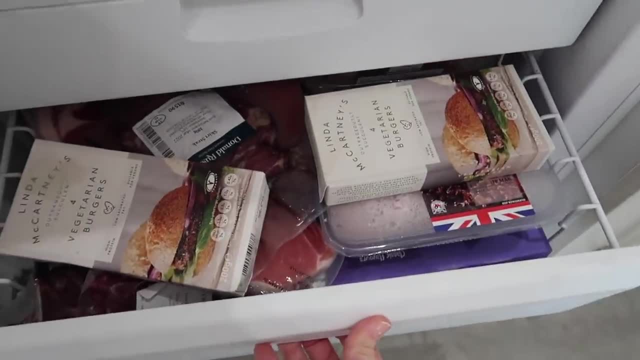 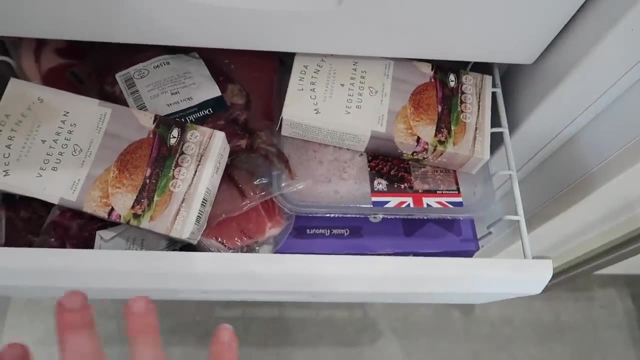 I've got peas. I've got lots of veggies and things like that- frozen veggies, And then in this bottom one I've also got meat. I've got some more pizzas down there, Yeah. so I've got quite a few bits in here, but I just feel like I could remove packaging and make everything fit a lot better. 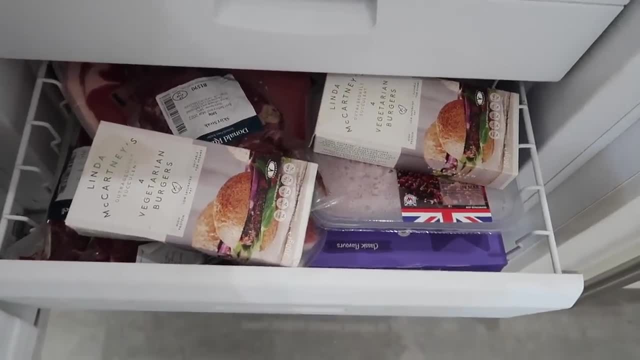 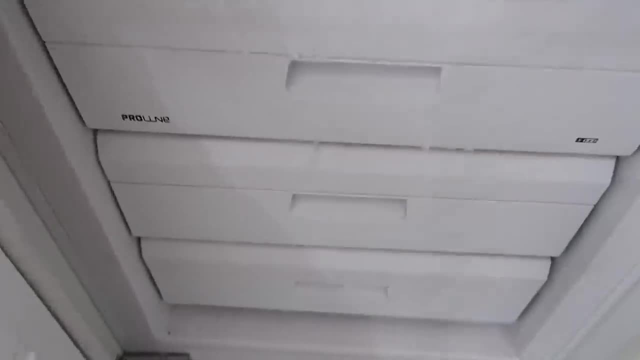 And also it's a bit of a mess, So I feel like I could kind of sort it out and put it into sections, So I know, when I open the freezer, exactly where to look for whatever I'm looking for. So it's now time to start defrosting and getting all of this. 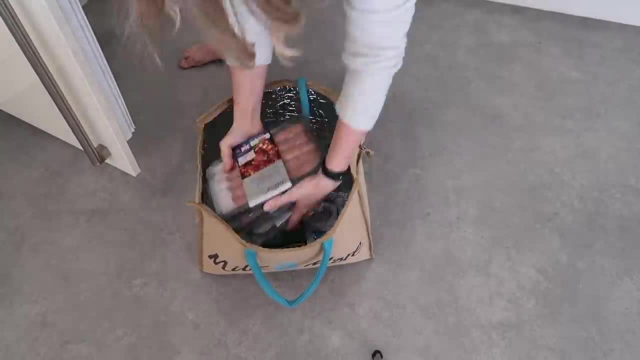 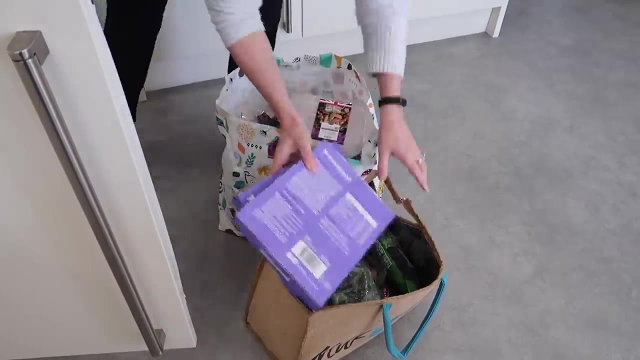 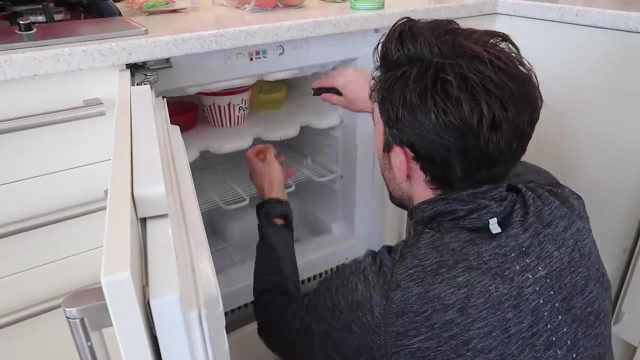 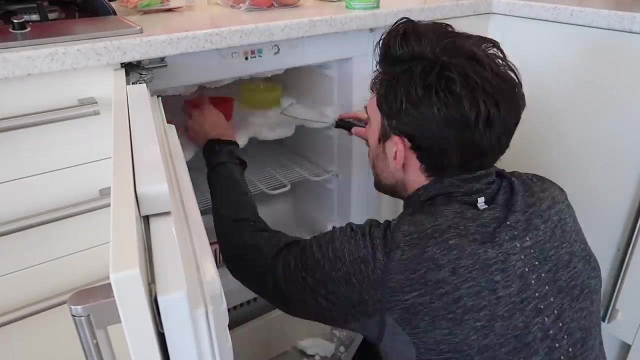 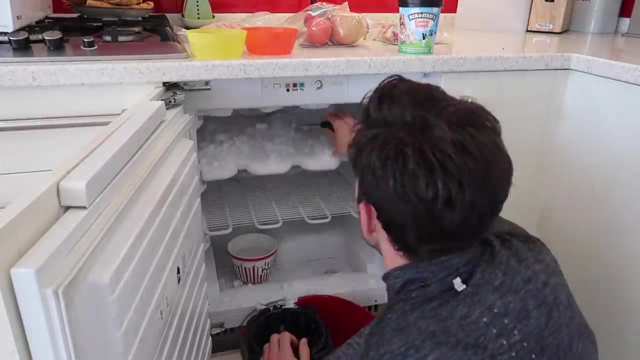 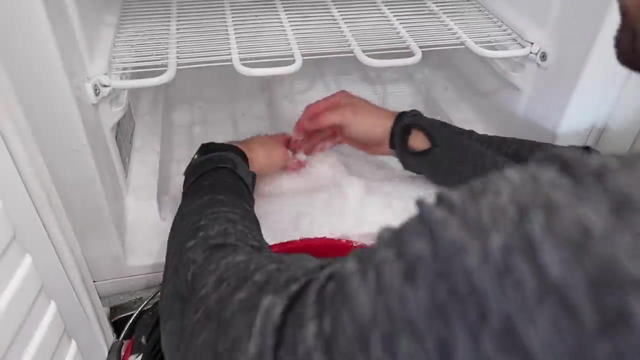 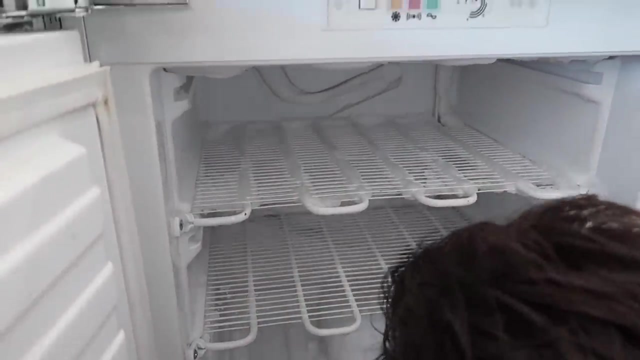 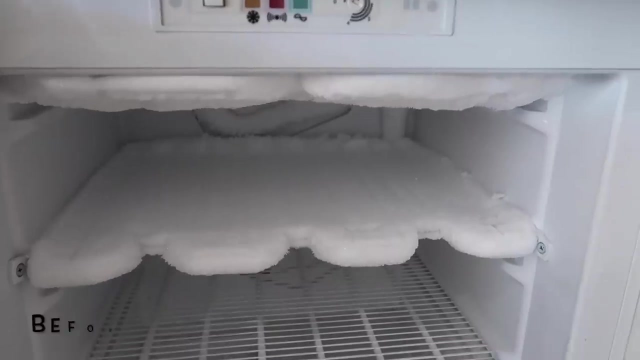 Ice off. So in this freezer obviously you've got drawers that go in. So you'd think like by taking away the ice it might not maximise your storage capacity, But our ice was like coming down so fast that even if you had stuff in your drawers you couldn't fill the drawers up to the top because 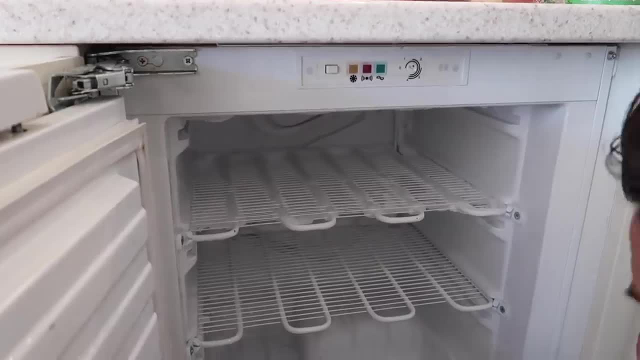 the ice would block it. So you'd have to fill the drawers up to the top because the ice would block it. So you'd have to fill the drawers up to the top because the ice would block it. So you'd have to kind of like three quarters fill the drawer. So this means we can now fill them right up to the. 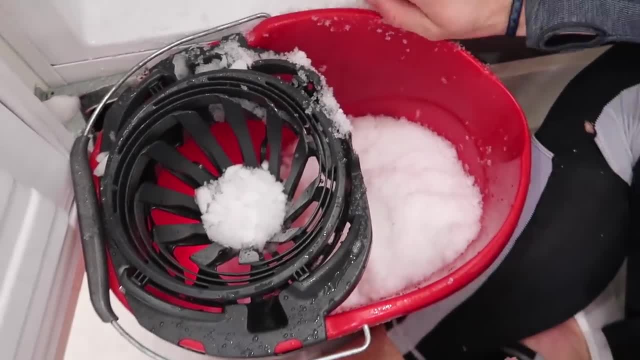 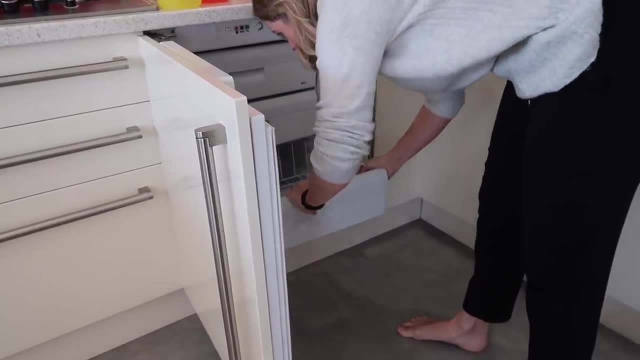 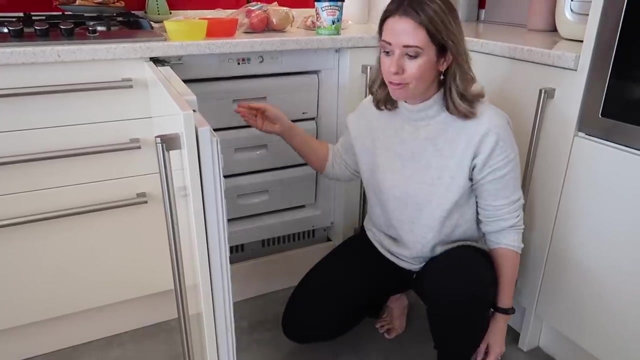 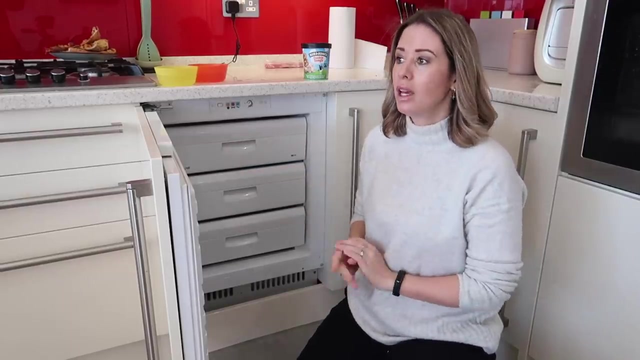 top. Wow, that's a lot of ice that's come up there. We can build a snowman. Look at that. Free and easy it goes in and out. So, like normally, your top drawer in your freezer would have your ice and things like that in. But 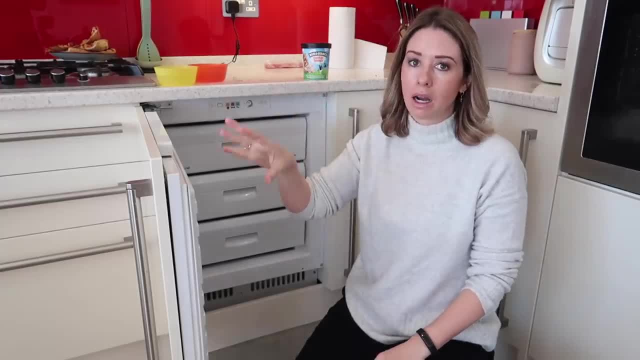 we don't really use much ice, So I've decided to just get rid of all my ice trays. I'm going to put them in the cupboard, So I'm just defrosting all the ice and then those will go away. And what I'm? 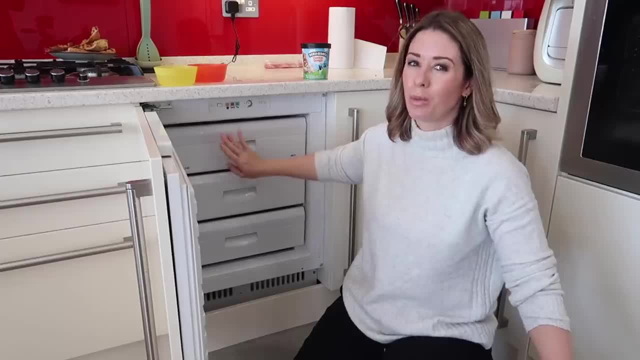 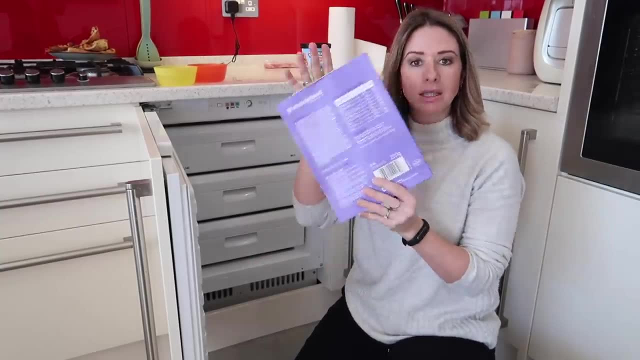 going to do is put in all my kind of fast food at the top here. So I'm going to put in all my pizzas, all my kind of like quick oven things, like the Linda McCartney sausages and burgers that I've got, But, as you can see, the pizzas come in cardboard boxes like this, and all the ones at Crispo as well. 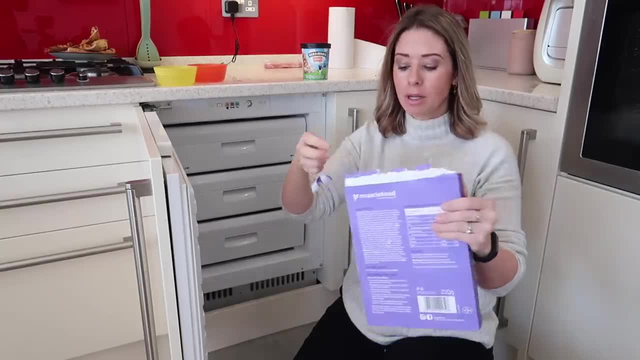 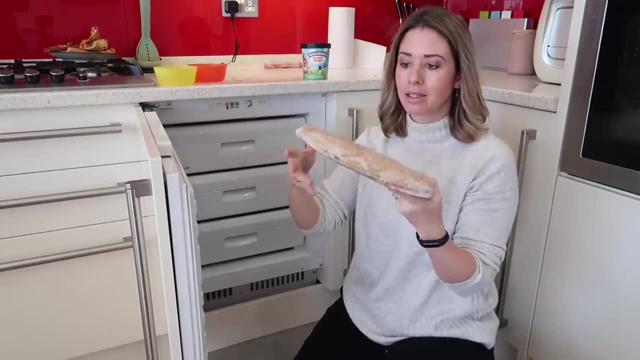 So what I'm going to do is just take them out of the packaging, because, even though they come in cardboard boxes like this, when you take them out of the packaging, they also are packaged in plastic, So the cardboard box takes up so much more space. 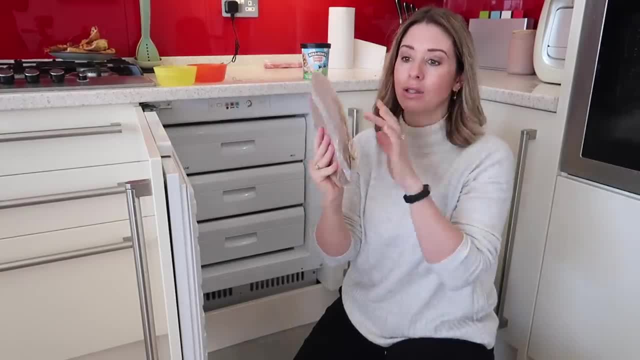 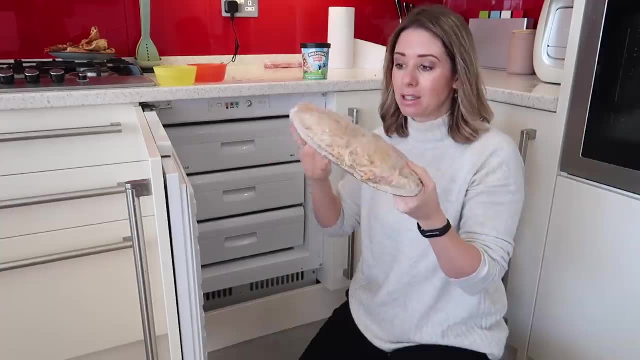 than just like without the cardboard box and the plastic in it, And obviously they're still kept completely like secure from having any like contamination on them or anything like that. So if you take them out of packaging and put them in your freezer like that, you're just going to get so much more in there. 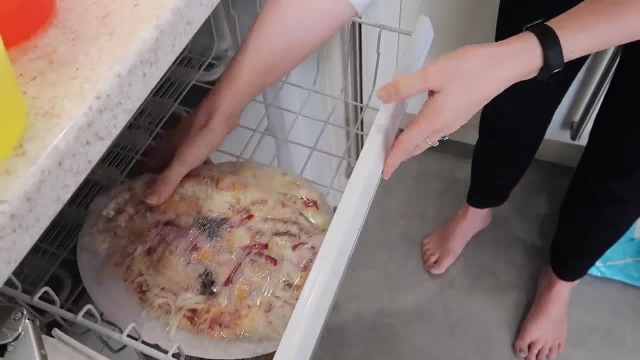 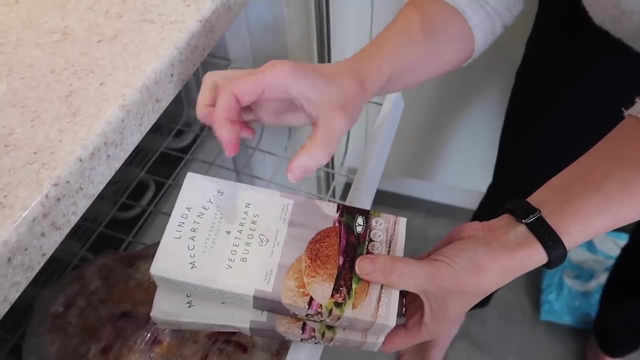 Music When it comes to cooking Music When it comes to cooking, to these Linda McCartney things. I'm actually not taking them out of the packaging because when you do take them out, they are individual, So I'm keeping these in the packaging. 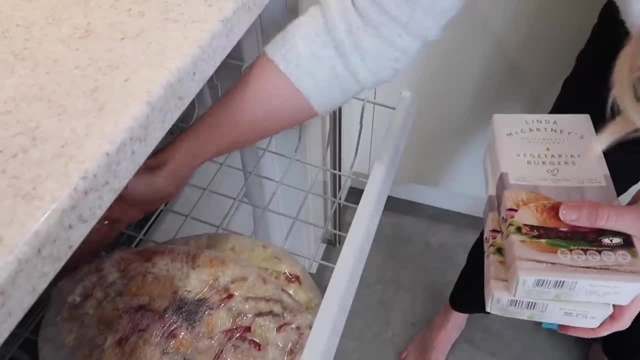 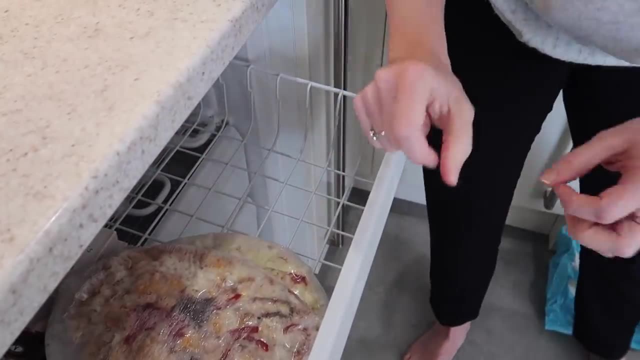 but because I have got so much more space without having like a big bulky box in here, I can just tuck these at the back there. I mean already I feel like that is so much more streamlined and so much better storage-wise. 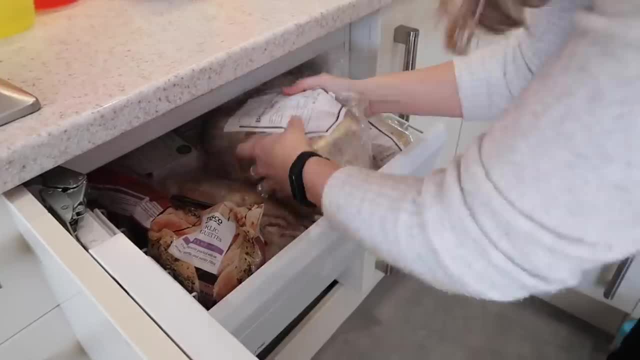 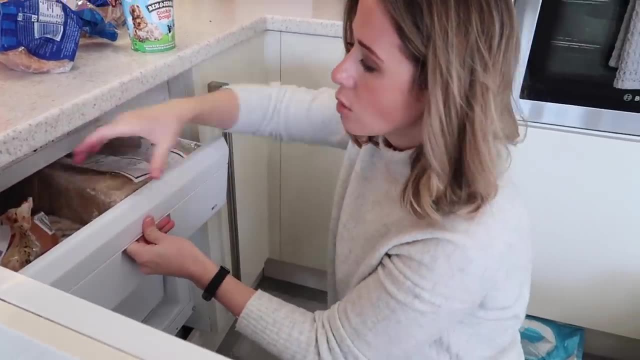 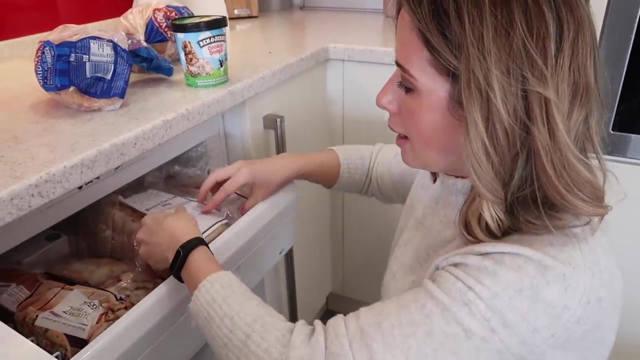 I can't fit like my bagels and things in there, but I've still got this little compartment here, So what I'm going to do is just fill up the other shelves and then I'll come back to this one, And I think I can get some more in there, but yeah, 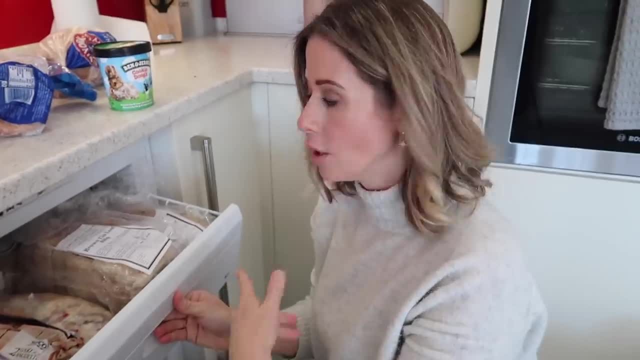 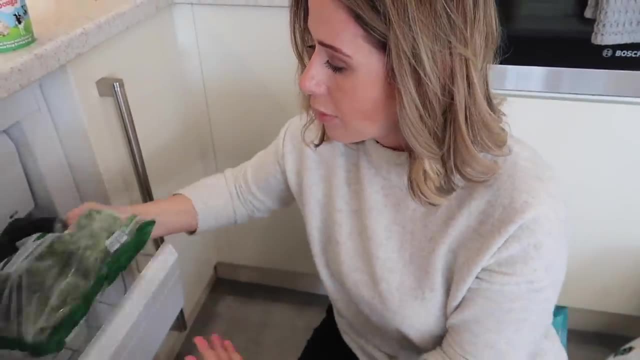 That I think before I defrosted it would have had to go in two drawers, Right, so bagels are going to go into my next one, along with some of my vegetables. These are all my frozen veggies. So what I try to do with the veggies- 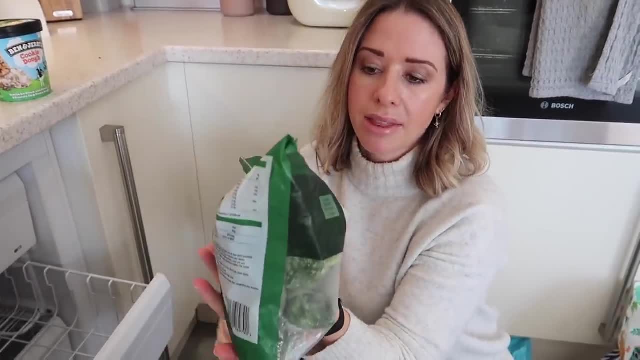 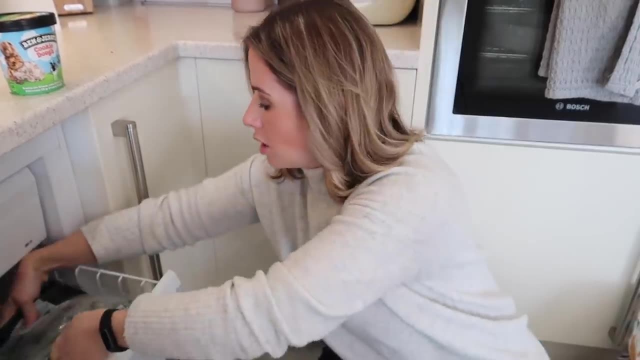 is lie them as flat as possible. If you just stick them in like that, they take up so much more space, Whereas if you give them like a large surface area, you can stack them one on top of each other. So I'll be putting these in and flattening them down. 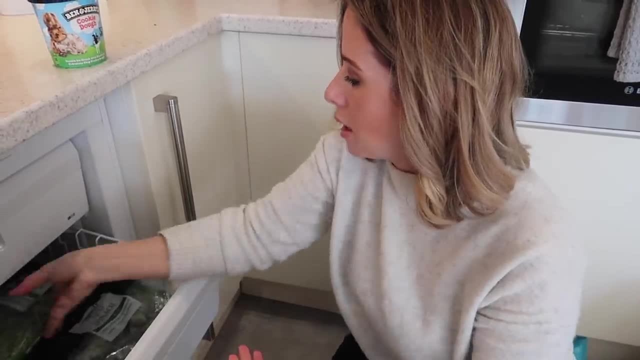 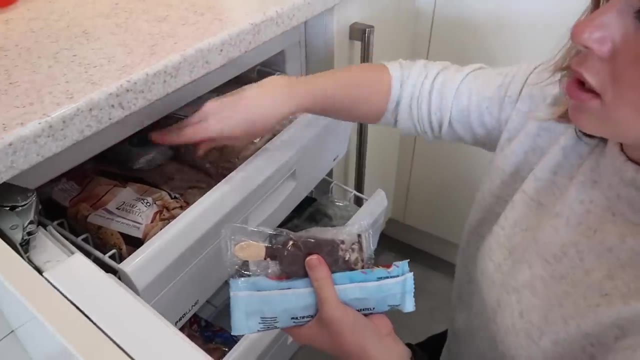 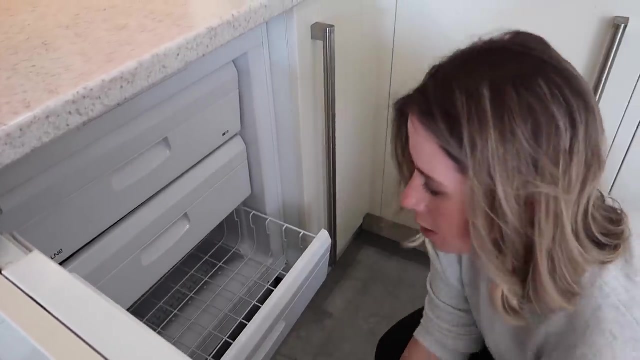 Nothing has defrosted while I've done this, So I've got my peas Again. flatten them down as much as possible All this time. it was never enough. All right, when it comes to my meat, I'm going to put all my meat at the bottom here. 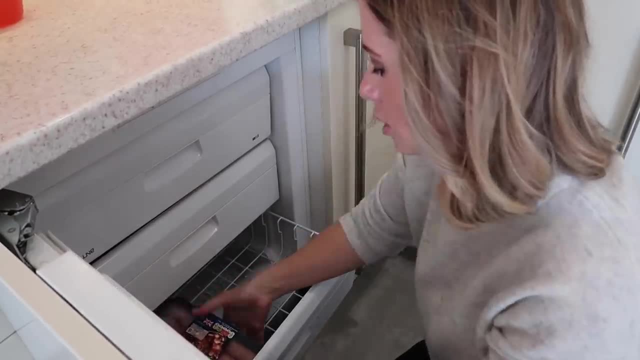 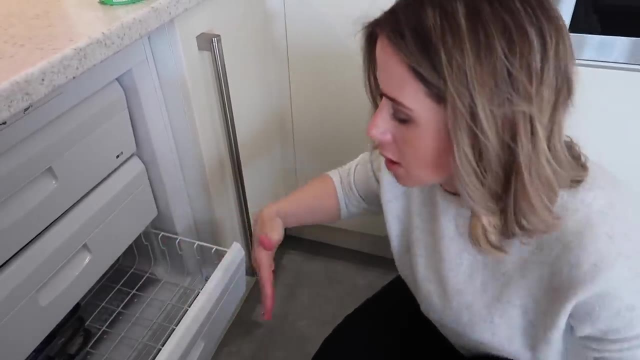 because you're actually meant to do that in your fridge. So I feel like if you're meant to do it in your fridge, you should probably do it in the freezer as well. So I'm going to start off at the back and just start putting everything coming forward. 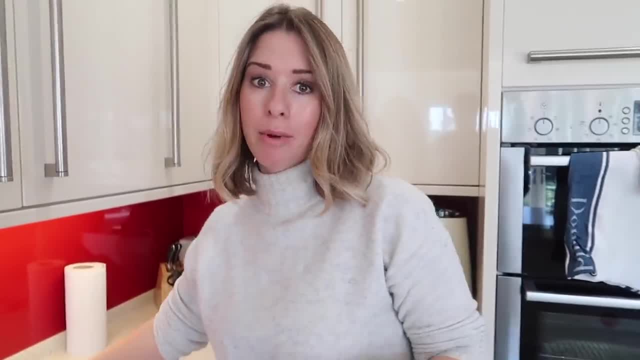 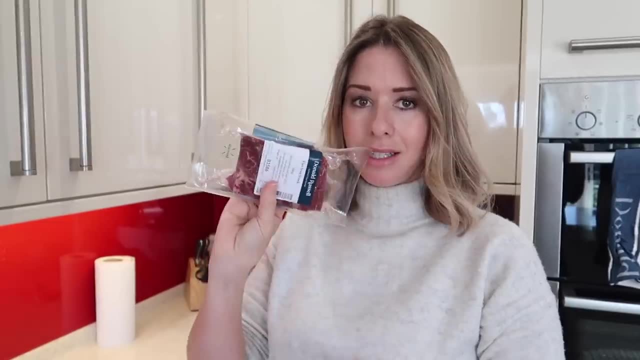 Ice cream. I wanted to show you a really cool tip for creating like vacuum packed bags. If you get a sort of Ziploc bag or a bag like this and you pop your meat inside. this is just an example, So this is actually already vacuum packed for me. 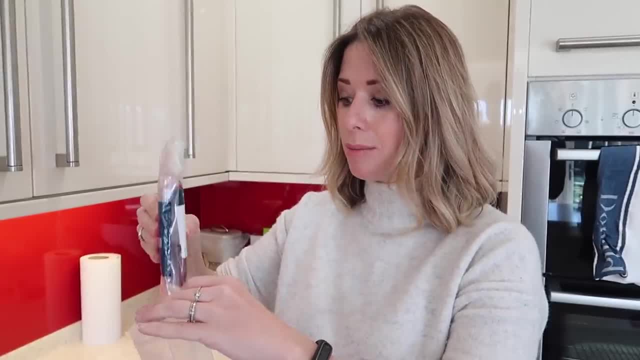 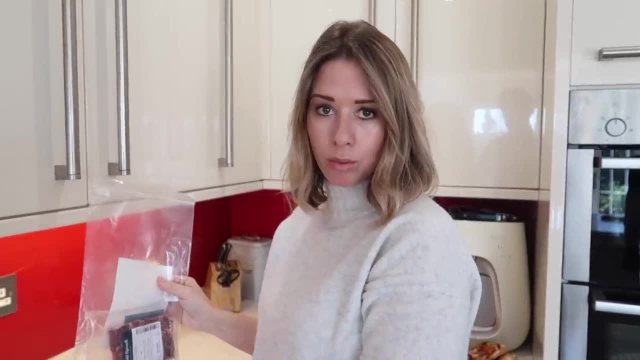 but I'm going to show you how you can vacuum pack yourself without having to buy an expensive machine. So you want to pop your meat into your little plastic bag and then get a pot of water and you want to dip your meat in the bag into the water. 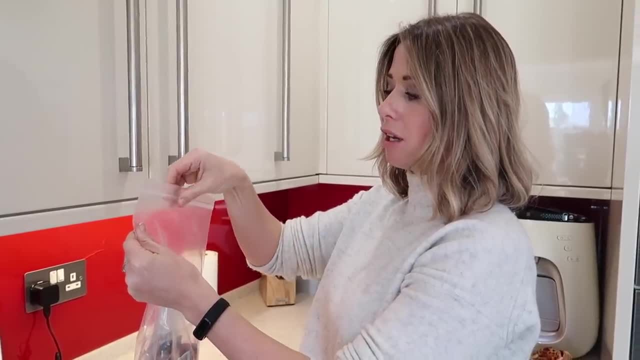 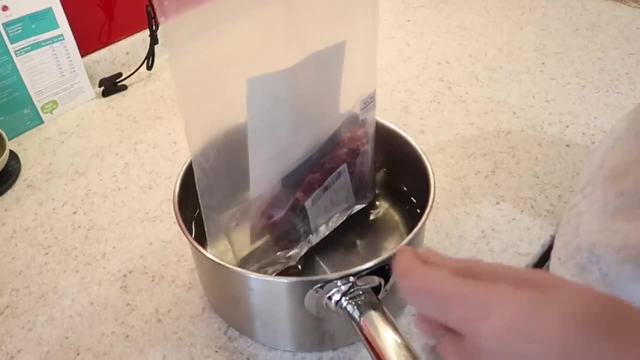 Just close up the top of your bag so it is nearly fully closed, but you just want to make sure you have got a little gap at one side so you can squeeze out the remaining air. Once you put your meat into the water, it's going to naturally push out all the air from the bag. 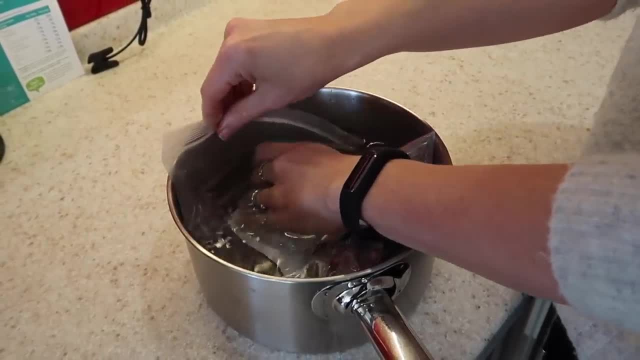 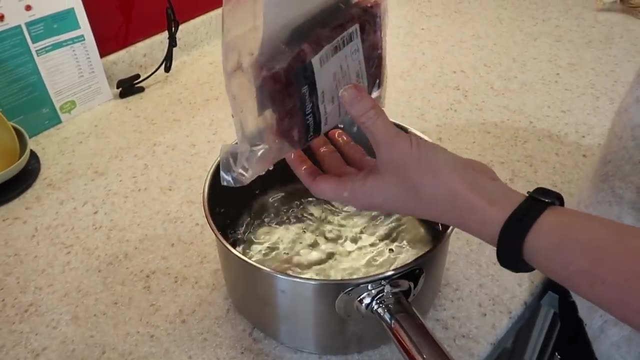 and just keep submerging it until you get to the very top. Don't submerge this bit, otherwise you're going to fill it up with water. Squeeze out every single last bit of air and then your meat is completely vacuum packed. This is a really good thing to do. 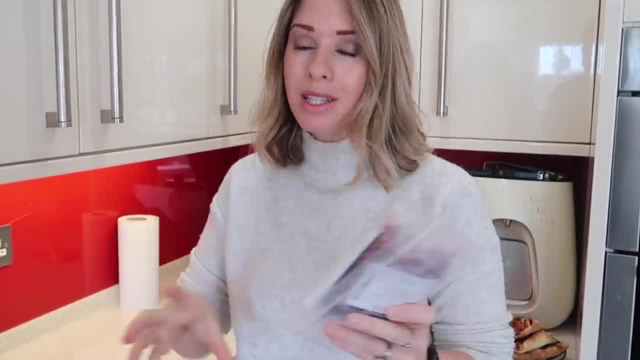 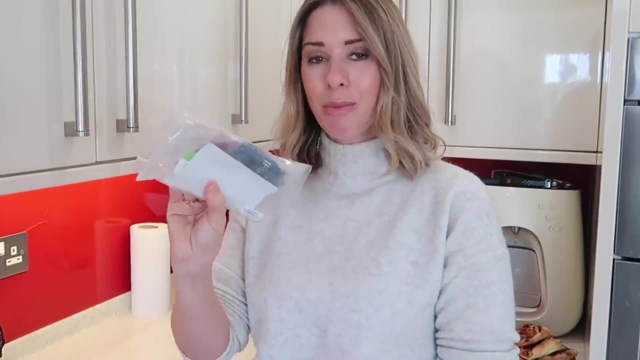 if you want to like bulk buy, so then you can separate all the different chicken breasts and things like that into portion sizes that you want. For example, we would probably portion it out as four chicken breasts in a portion Vacuum pack- each four lots of chicken- and pop them. 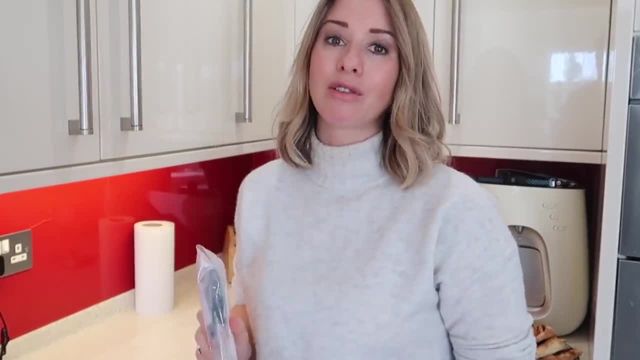 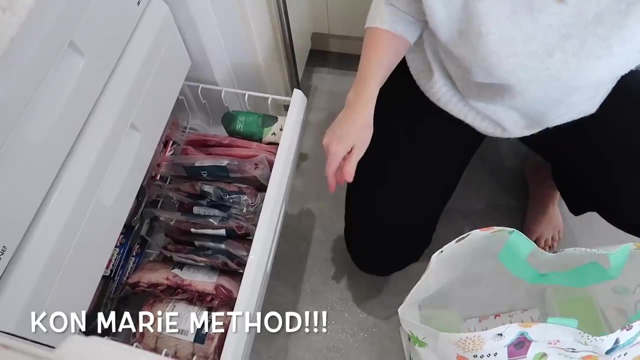 in the freezer like that. That way, you're going to make sure that when you get some chicken out of your fridge, you're going to have just the right amount that you need to feed your family. That's everything back in there, but I'm going to put some more meat. 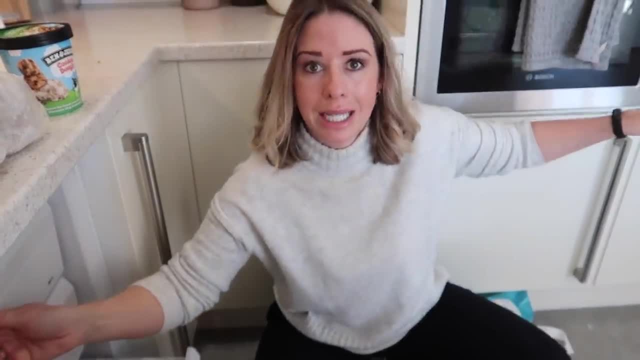 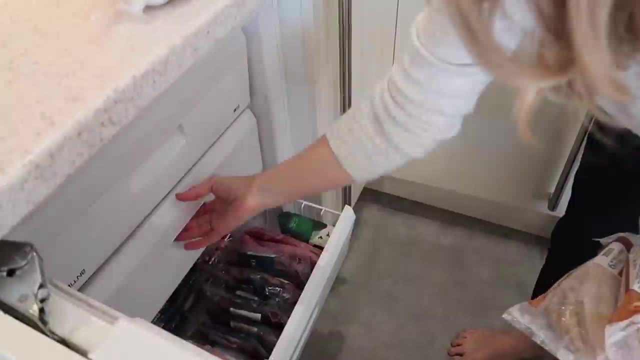 from the other freezer now into here as well, because I've taken my bread out of that freezer and put it in the top two shelves as well. So I'm going to see if I can get even more into here from that one. It was never enough. 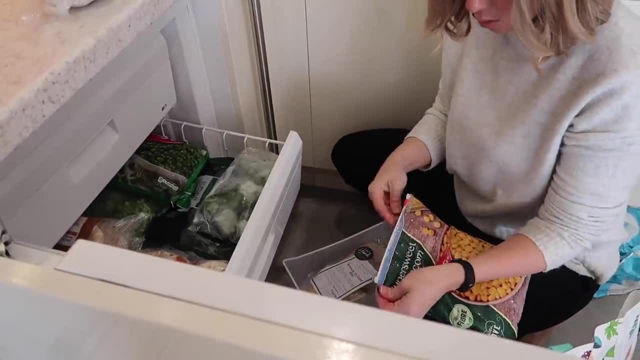 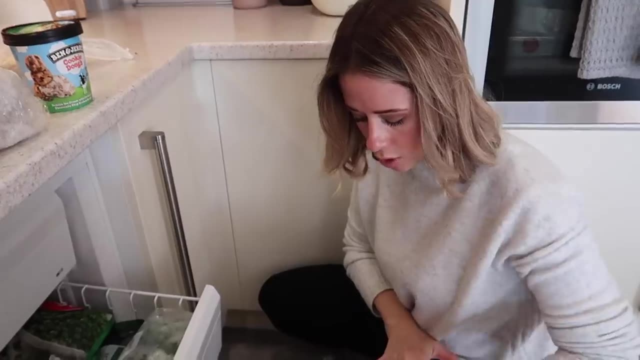 Also, when you've got your veggies like this, I've just like broken them all up and I've laid them flat. I can feel there's quite a lot of air in there, So I'm just going to undo the little bit here and just press out as much air as possible. 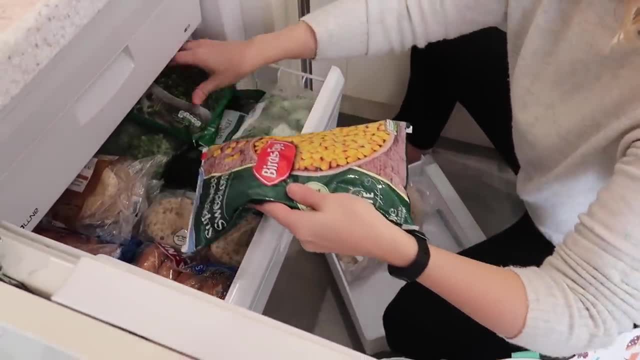 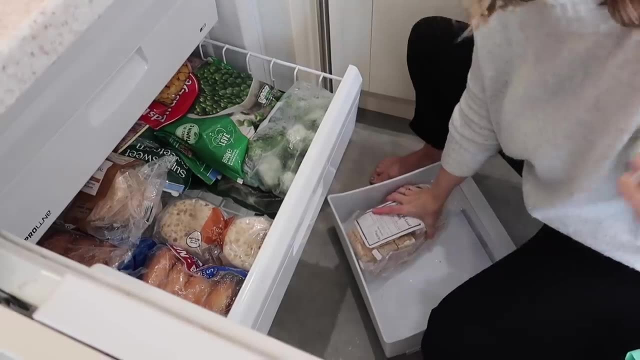 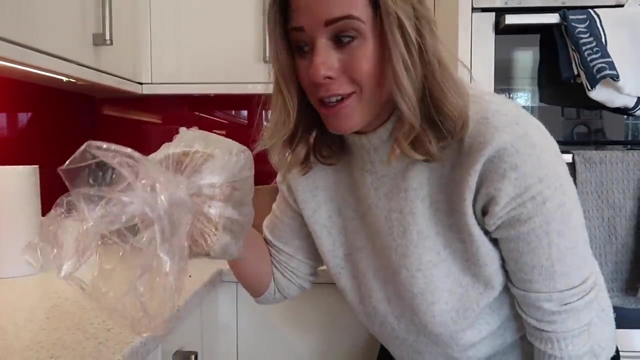 And then it just works out to be so much butter. Oh my gosh guys, I've got that whole freezer that's free. I've literally got that left from the other freezer. Come over. I mean, this needs a really good, clean, but look. 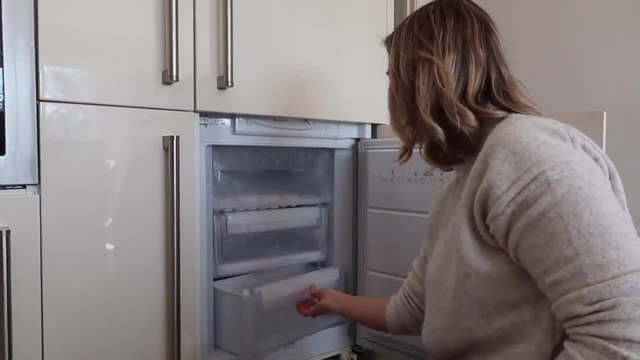 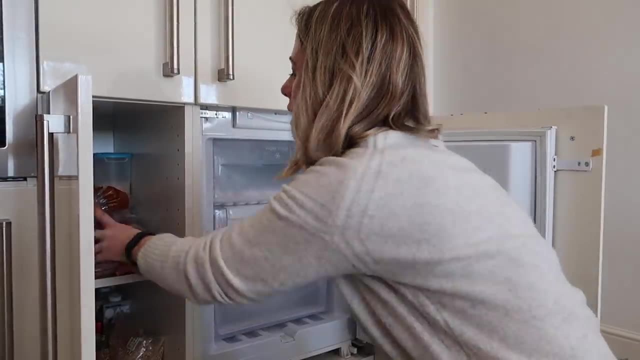 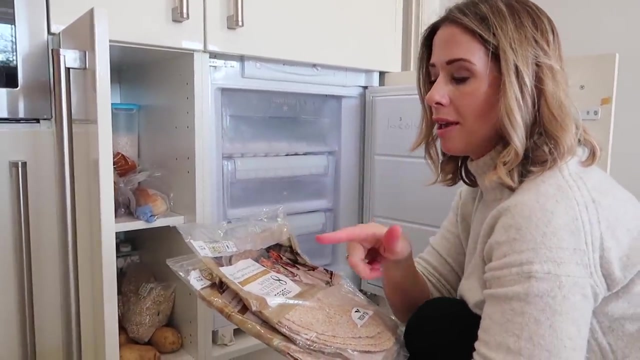 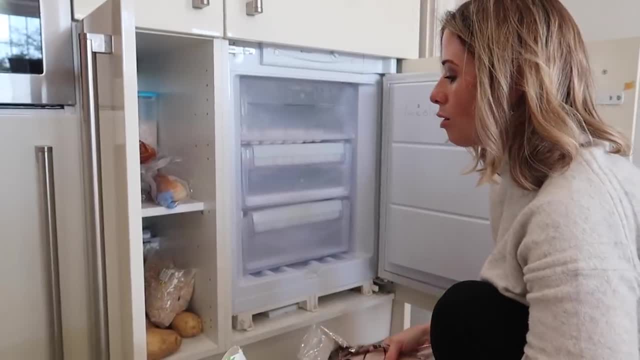 Now I've got extra space, I'm going to freeze these as well, So I'm going to go through my cupboards and see if I need to freeze anything else, Right? so here is my second freezer that has been fully defrosted. 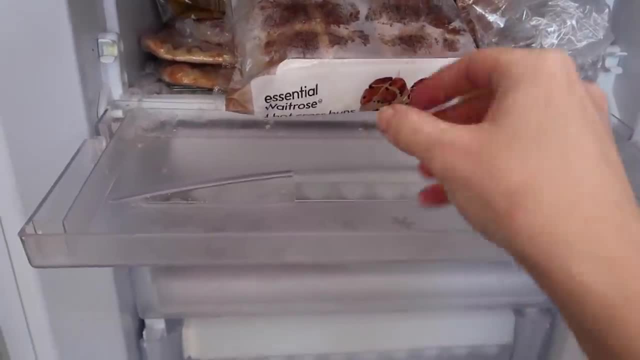 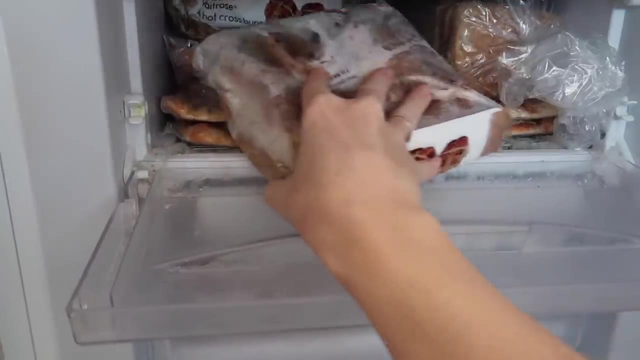 and we've also put some extra supplies in here. Chris got, like I said earlier, he went to the shop and got a few more bits. We've got some hot cross buns, more pizzas in here, because that's what I just saw him come home with. 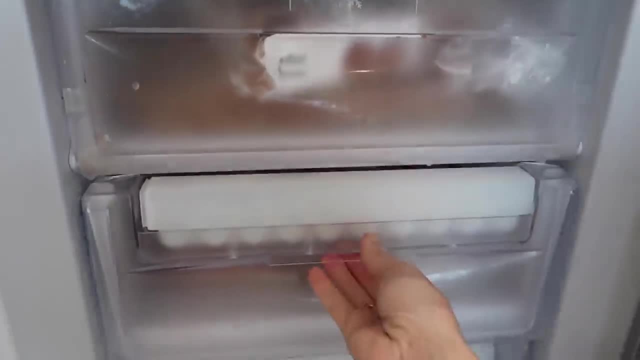 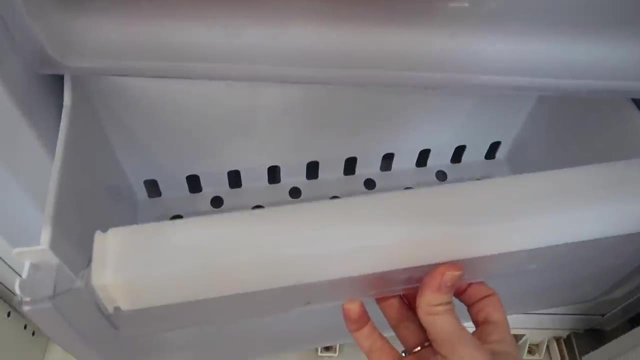 And then we've also got some bread that wouldn't fit in the other freezer In this drawer. we have got some chips and some more corn burgers, And then we have got a whole freezer. So that's it, That's it, That's it.